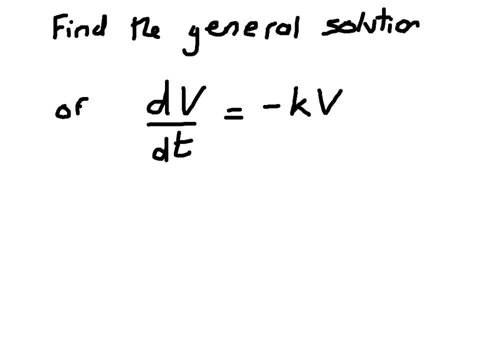 So I'm just going to look here at how we'd solve this. The most important thing to remember is separating the variables before you solve. At the moment, I have v and t on the same side of the equation, and that simply can't happen. 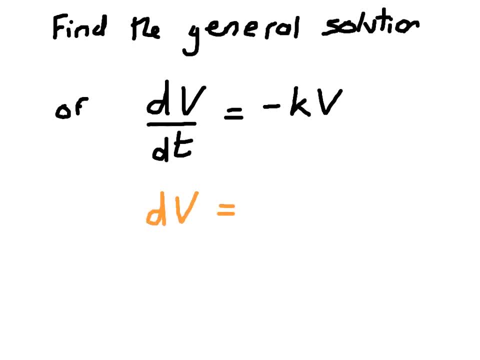 So what I need to do is multiply the dt up to get rid of it. But now I've got a problem with that big capital V over there on the same side as the dt. Now I can divide by minus kv. I could just divide by kv. 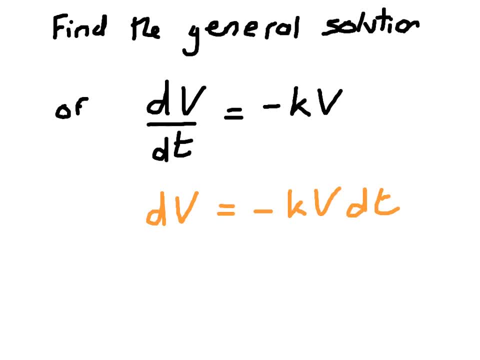 Or I could just divide by dt. The most important thing is, we can multiply and divide. It's very rare to use subtraction and addition. I will show you one example of that in a few moments. So what I'm going to do, I'm just going to divide down just by the v. 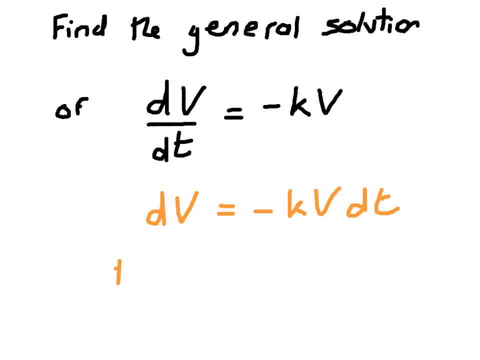 So on the left-hand side I have 1 over the v. dv equals to minus k dt. And now, once you've got all the v's on the table, you're going to have to divide by v. So if you've got all the v's on one side, all the t's- there weren't many on the other side- then you can integrate. 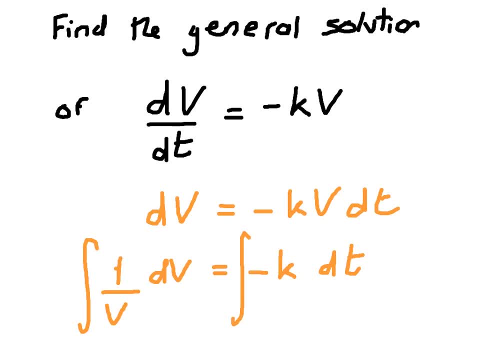 Now, this isn't a tutorial on integration, And often people say I'm struggling with differential equations and what they mean is they can't integrate, And that's for another time. but do make sure your integration is sound. The integral of 1 over v becomes the natural logarithm of v. 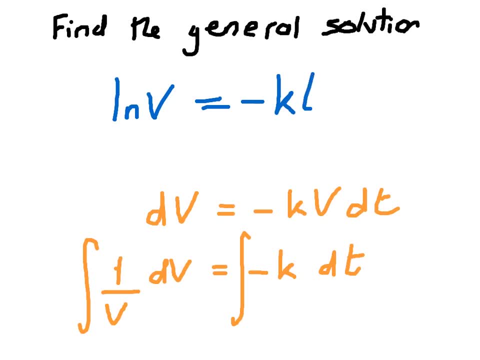 And if we integrate minus k, we get minus kt, Because minus k is just a number Plus c. That's the general solution. We haven't found what c is, but you don't need to for the general solution. Let's look at a question where we do need to find what c is. 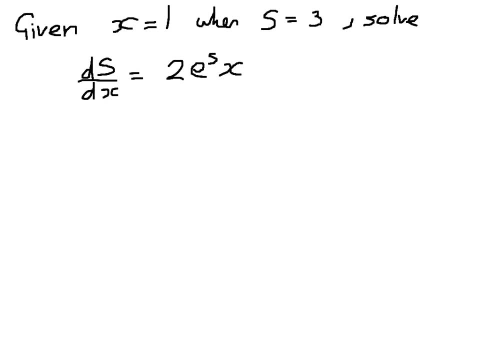 Now in this question we're given some information and we're just told to solve the differential equation. And you see that solve. you know you're going to have to separate and integrate And then we'll use the information in a few moments. 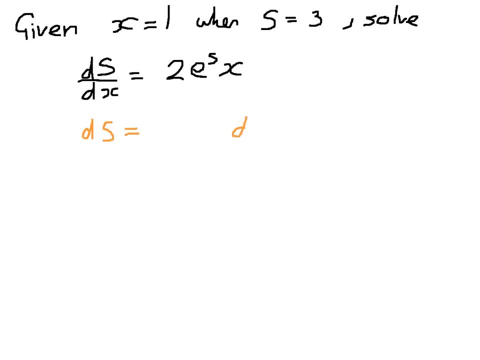 So you can see that I can multiply the dx up, I can put it on, I can put it on this side, and that would leave me with the x there. That's great, And I could leave the 2 there, but it doesn't matter which side you take it. 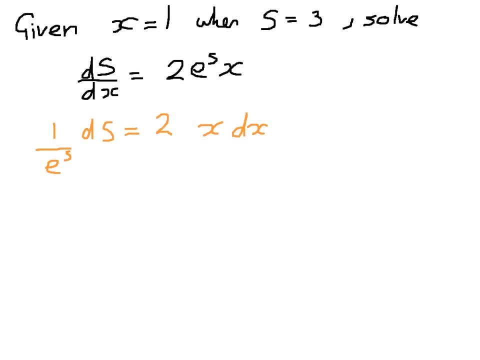 But I need to divide through by e to the s. I've got all the s's on one side, all of the x's on the other, So at that stage I can integrate. Now you can't integrate 1 over e to the s just as it is. 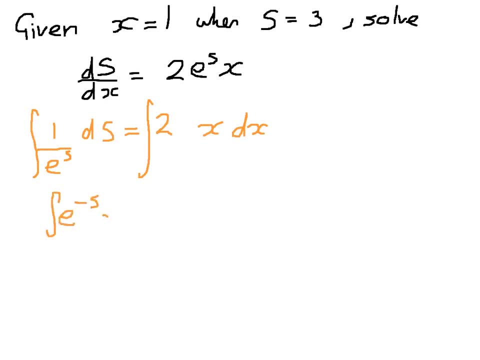 You need to consider the fact that you're integrating e to the minus, s with respect to s, And you're integrating 2x With respect to x. Now again, if you're not sure how to do that, it's not differential equations you have a problem with. 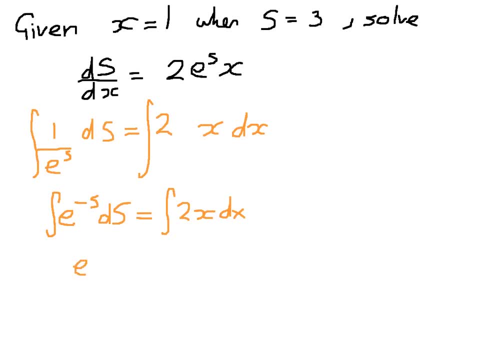 It's integration, so make sure you revise that thoroughly. This becomes e to the minus s, all over minus 1. And this side would become well 2x squared over 2.. I need to cancel them out, Plus c. 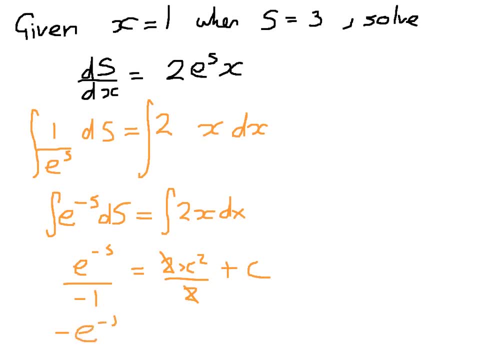 Now I could just write that as minus. So I have minus e to the minus s equals x squared plus c, And that's my general solution. But in this question we weren't asked for the general solution. We were asked to solve. 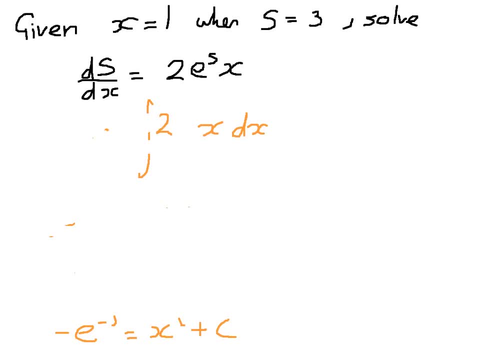 And so it's at this stage that we need to use the information that we've been given. So what information do we know? We know when x is 1, then s equals 3. And we're going to substitute these in. 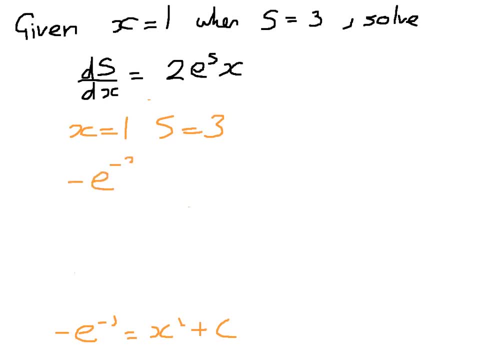 So I have minus e to the minus 3.. Equals 1 squared, which is just 1 plus c, And rearranging that, you can see therefore, that c equals minus 1, minus e to the minus 3.. So we now know what c is. 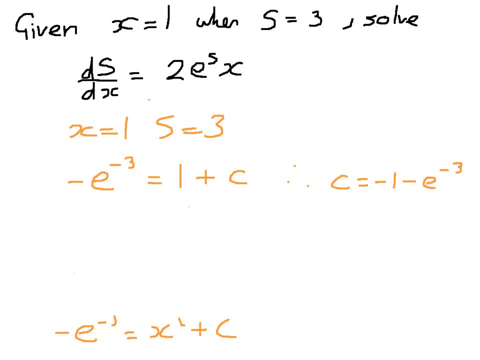 The question wasn't find c, It was solve the differential equation. So my answer is minus e to the minus s equals x squared, And then c is minus 1, minus e, Minus 3.. They didn't ask me to say find it in the form s equals. 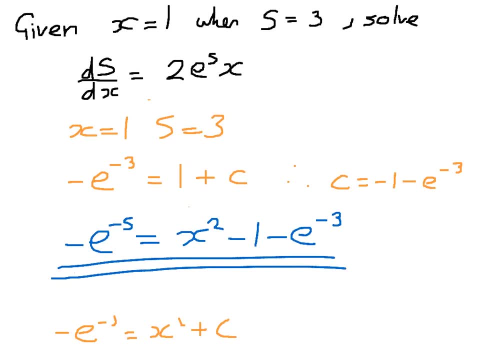 They didn't say find it in the form x equals. So if they don't do that, you simply get to this stage. But do bear in mind you may be asked, of course, to rearrange it, to say s or x equals. 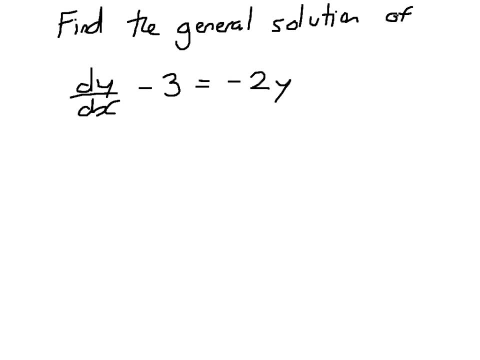 Now let me just show you one or two tricky examples. Now it's worth pointing out that I've never seen it asked this way in a C4 A-level examination. I have often seen it in some IB higher examinations. But it could come up in either. 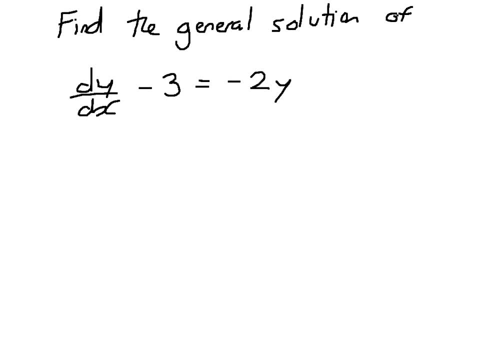 The material is exactly the same as what we've been doing. We have a differential equation. Now I don't want to multiply up by dx at this stage, Because if I did, then obviously I'd get the 3dx and the 2ydx. 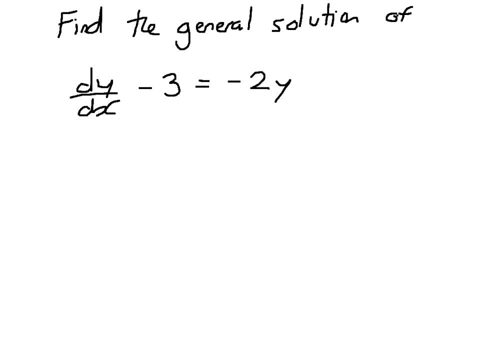 So, before you do your separation and solve, that's when you want to get everything on one side. So I'm just going to move that 3 over to the other side, where it becomes plus 3.. Now, normally, once you get to this stage, I say: do not do any further addition. 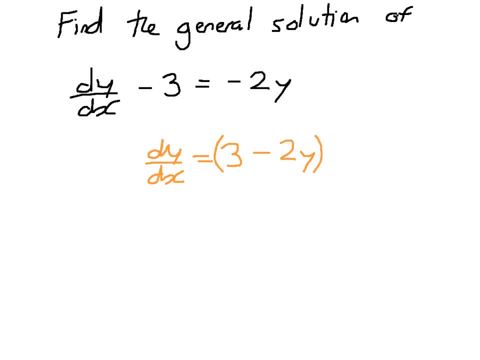 Or subtraction. And the reason for that is when I multiply up by the dx, it kind of all gets multiplied by that now. So the dx is going to go with all of this And this gets locked together. So the point there is: make sure you get your derivative on its own on one side. 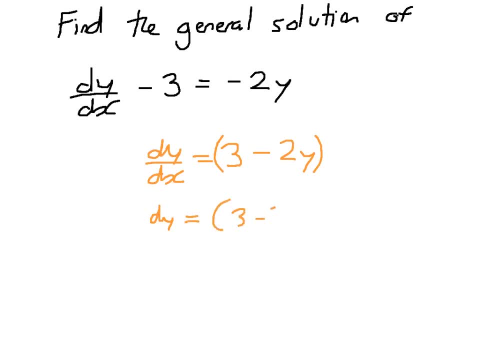 And at that stage you can multiply up, So 3 minus 2y dx, And then I can divide down. I can write that as 1 over 3 minus 2y y equals. So there's nothing left. There is a 1 left. 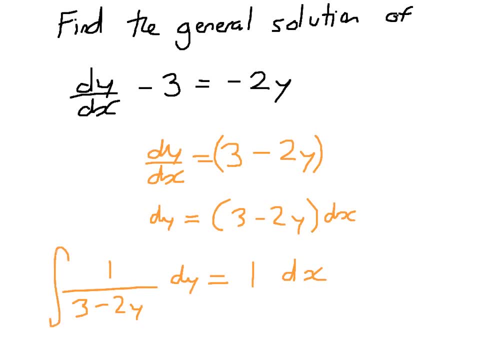 People often forget that dx, And it's at that stage that I can integrate. Now I've said it several times today: If you struggle to integrate that, it's not differential equations you have a problem with. You're probably awesome Or you're going to be awesome at differential equations. 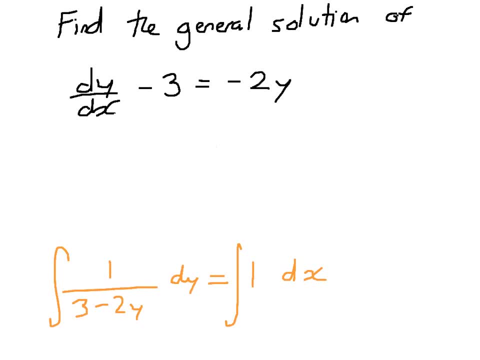 It's integrating. That's what you need to practice. So watch further tutorials and work on that. This, and you should see, becomes well. it's not because it's on the bottom, It's because it's on the bottom. 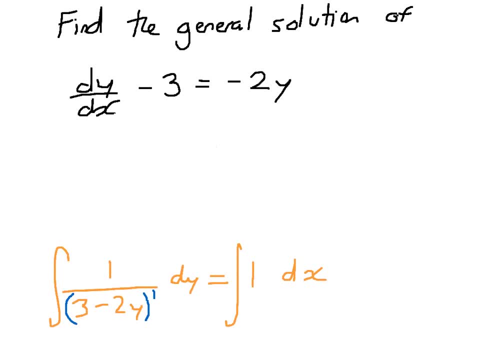 It's on the bottom, to the power 1.. So if I didn't write it on the bottom it would be to the minus 1.. You should know that that becomes the natural logarithm of 3 minus 2y. If I was differentiating that, you should know that using the chain rule, I'd times 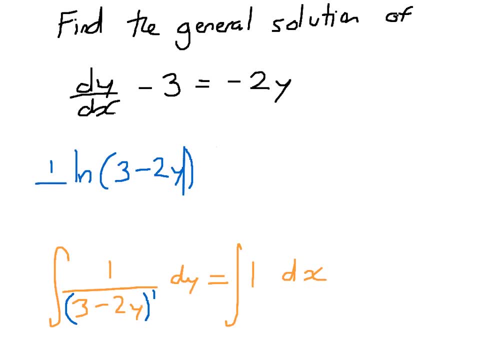 it by minus 2.. I'm integrating, So I'm going to have a minus half at the front. That equals 2. And this just becomes x plus c. There is your general solution. If you had information, you could go on to solve this by finding c. 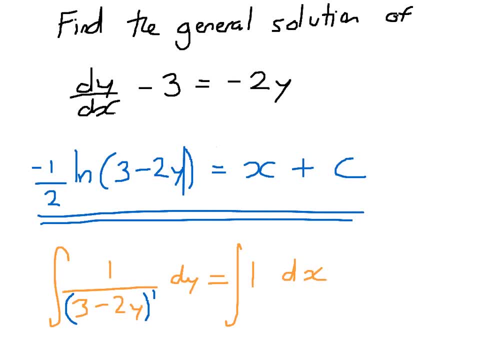 I could rearrange this into the form y equals very easily, or x equals even easier, But the process is the same: Separate then solve, Separate, then solve. And if you practice your integration, you'll be able to solve any of these integrals. 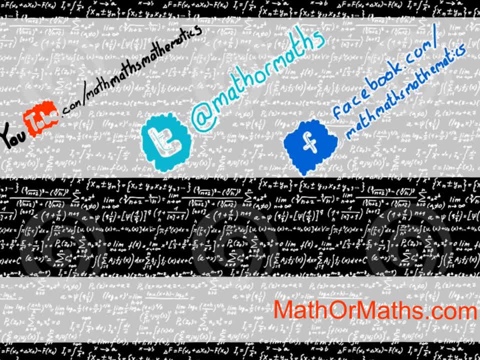 So really good luck with that. If you need any more help, visit mathallmathscom and do request videos. This was requested by Bex. I really hope it's helped, Bex, And I know you're going to do awesome in your examination. 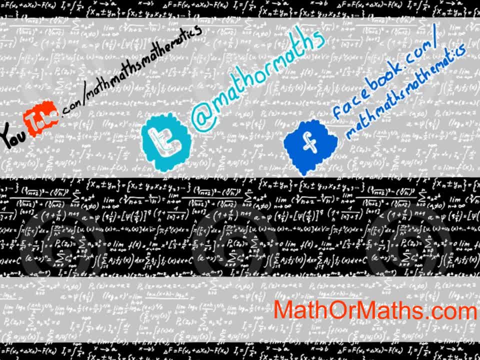 Follow me on Twitter and check out my Facebook page for updates of what I'm doing, And please share this with your friends. They really will appreciate it if you help them in their examinations, And I really appreciate being able to help more people. I hope I've helped you. Good luck in your exams. 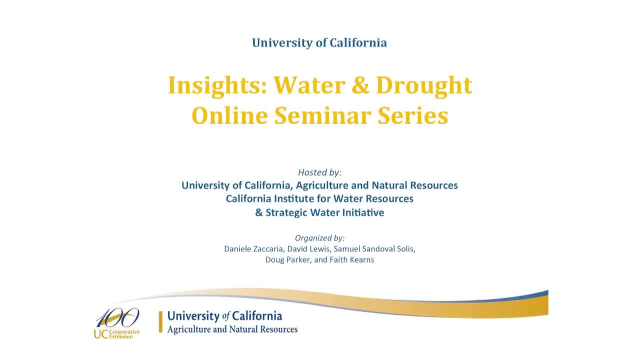 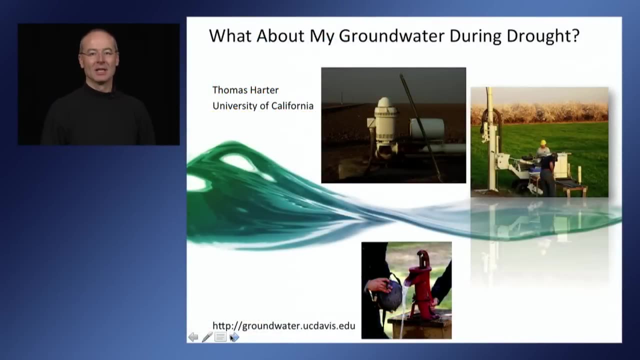 Hello, my name is Thomas Harder. I am faculty and Carburetor Extension Specialist with the University of California at Davis. With this video, I want to talk about groundwater and maybe explain a little bit about what may happen to your groundwater during this drought, or any other year for that matter. 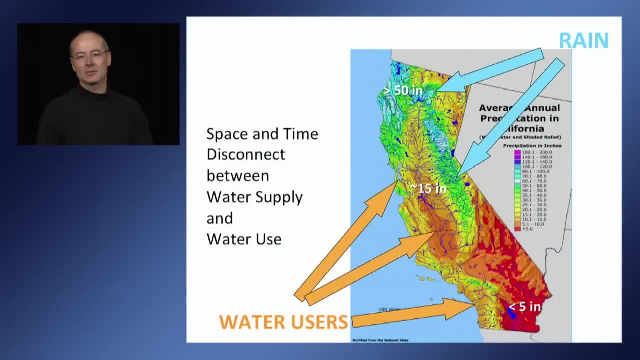 California has a fundamental problem with water. We have both a temporal, a time disconnect and a space disconnect between where we have water available, that is, where it rains, and where we actually use the water. If you look at this map, you can see that most of the rain falls in Northern California. We have places with more than 50 inches of rain in a normal year. 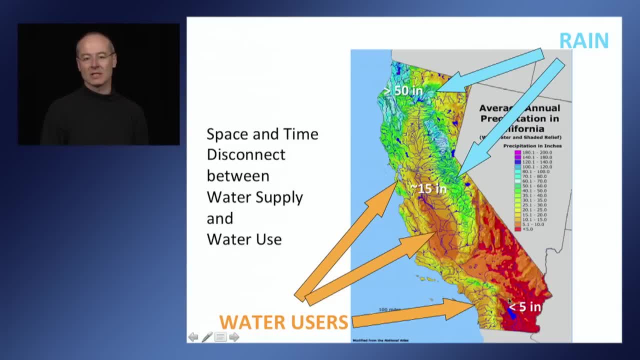 But most of us use water in the central part of California and in the southern part of California, where we have 15 inches of rainfall and down in Southern California less than 5 inches of rainfall. What we have done to both bridge the temporal or time disconnect and the spatial disconnect is we have built storage reservoirs that help us save the rain that falls in the winter for use in the summer.